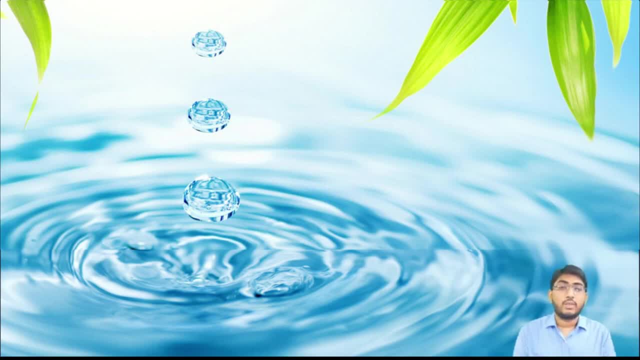 it is mandatory to treat it before supplying to the consumers, Right? so in today's video, we will discuss about the next topic, that is, the water treatment processes and treatment units. Okay, so which are the different processes that are present in a water treatment plant? 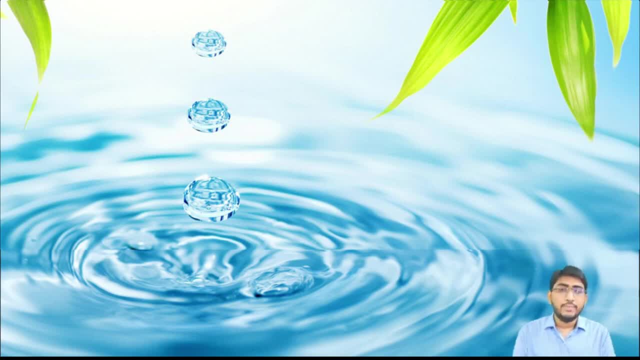 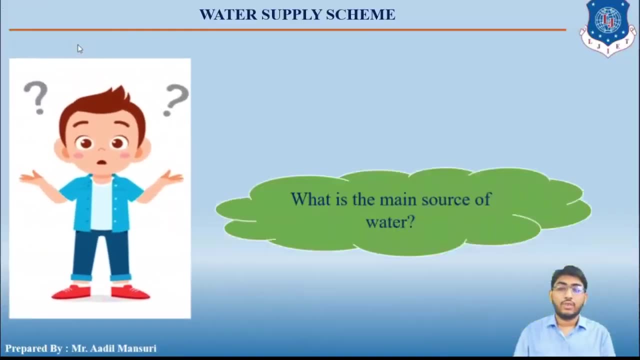 in order to remove various types of impurities. Okay, here are the activities involved, including tonight's part. Let me ask you the first question, that What is the main source of water? Okay, so the answer is: the main source of water is rainfall, and we know that it is the purest form of water. 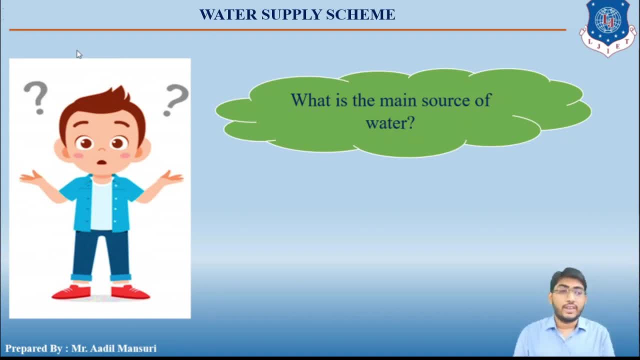 So you might have now a question that since rainfall is the purest form of water, then why do we need to treat it right? So The precipitation occurs in the form of rain droplets. it passes through the atmosphere. okay, so it. 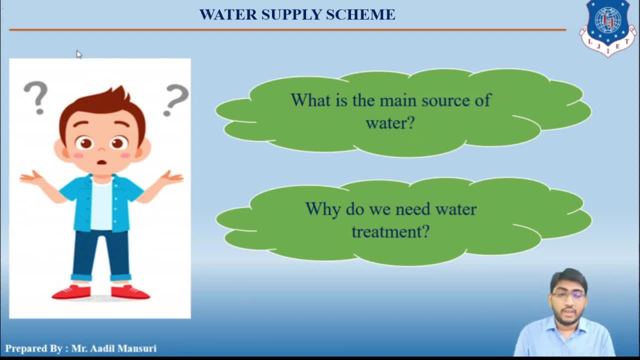 may dissolve certain gases, traces of mineral matters and other substances, and thus it is possible that it may get contaminated while reaching the earth surface. okay, so, therefore, surface water is required to be properly treated before supplying to the consumers, and this treatment takes place at the water treatment plant. okay, understood, students? so main source of water is rainfall and 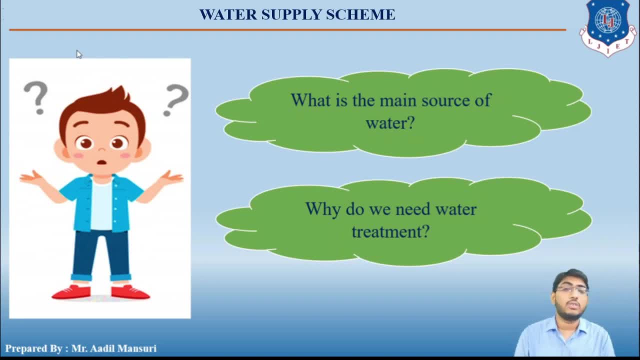 because it passes through the atmosphere, it dissolves various impurities, and when the water gets accumulated in the surface sources and when we extract it, we need to treat it before supplying to the consumer. so let us move ahead now. what happens to the water after precipitation? okay, so now some portion of rainfall. 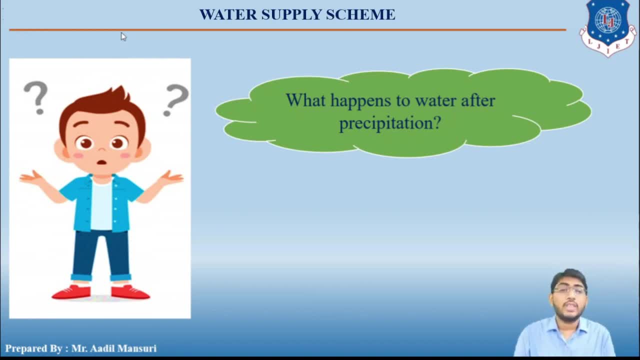 percolates into the ground and it follows the action of filtration and thus groundwater is free from suspended impurities and bacteriological impurities- okay, it may be present sometimes also. now the groundwater can be directly supplied without treatment and only disinfection is done if the 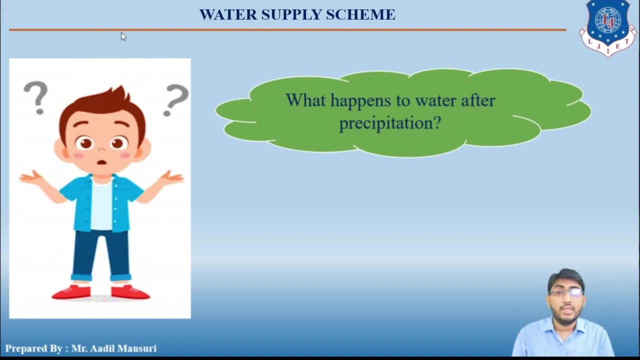 dissolved impurities are within the permissible limit. now the surface water source is the only adequate water source to supply the water to the large communities as it is available in abundance as compared to the groundwater. okay, as all the amount of groundwater cannot be extracted easily or economically okay. so I hope you have understood about the 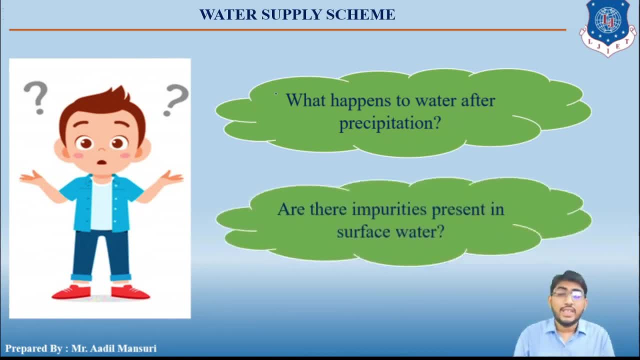 surface water source. so now let us move ahead. so the question is: are there impurities present in surface water? so yes, the surface water contains high to low amount of turbidity. that is, varying from 500 to 90 NTU, which stands for nephelometric turbidity unit, and also high amount of bacteriological 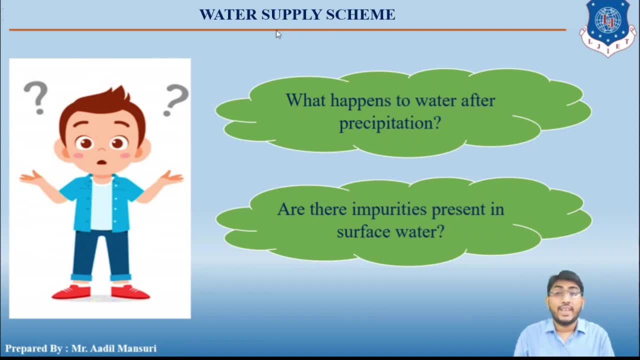 impurities with other impurities in varying seasons. okay, so, as we know that in monsoon season, when the runoff takes place from the catchment area, it takes with it lots of surface loads, right, so this impurities varies from season to season, okay, it is therefore very essential that, to satisfy the 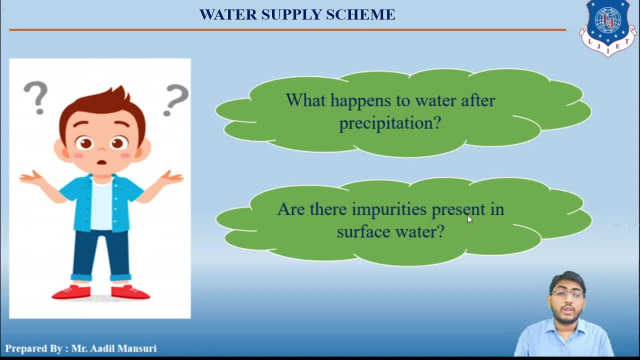 characteristics of wholesome water. surface water needs to be treated before it is supplied to the community. okay, students, and the amount of water is very whole. sub water needs to be treated before it is supplied to the community. ok, students, and the amount is. very. concerned about what we hope is needed after this. we call into 2019. we need the ratings for the span of landmark in the month born: 34 א linght, in which number of mieve weightlands- this is nita 6시는- is given by the country and number of municipalities. industries are required to be treated before it is played by the community. previous year results related to the canada educating various parameters of today students and the 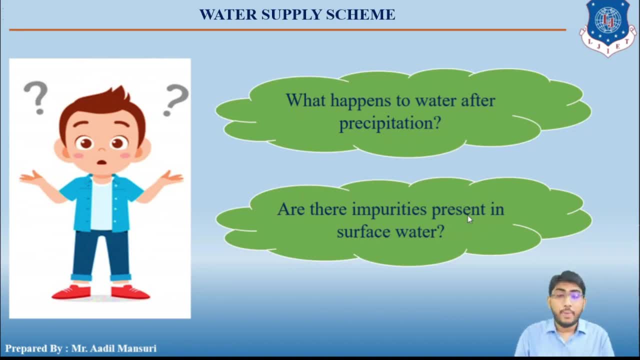 amount and the type of treatment process will depend on the quality of raw water and the standards of water quality required after the treatment. okay, so which treatment is needed depends on the test which has been done in the laboratory and even after treatment. whether the impurities are in permissible limit or not. it is checked before the supply, then only water is. 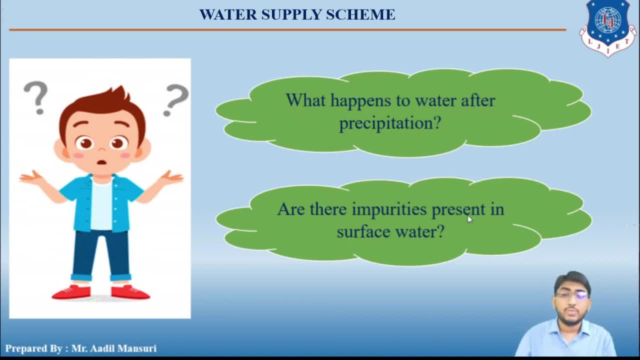 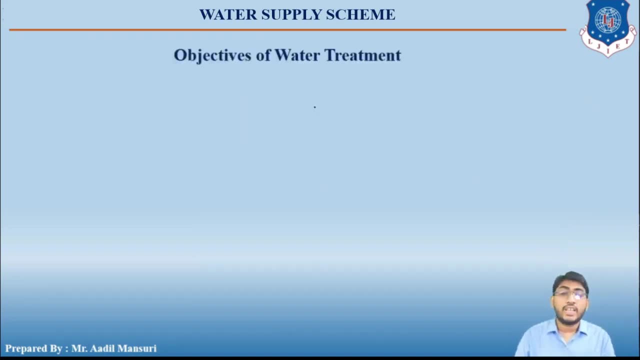 supplied to the community. okay, so let us move ahead, students. so let us now talk about the objectives of the water treatment. okay, so the main aim of water treatment is to produce and maintain water that is hygienically safe, aesthetically attractive and palatable in. 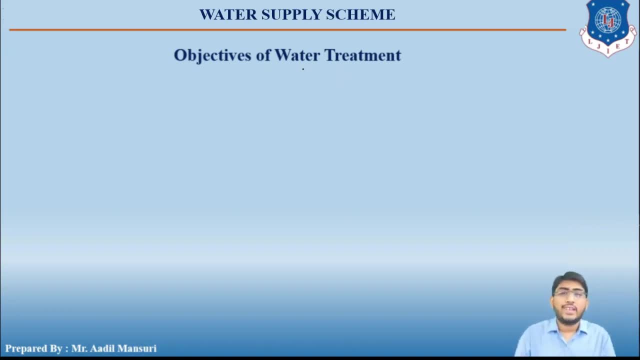 economical manner. okay, so we all know that, after extraction of water, water is used to produce and maintain water that is hygienically safe, aesthetically attractive from the different sources. it may contain different types of impurities, okay, and so after treatment, the water should be hygienically safe and it should be looking clear. okay, crystal clear. 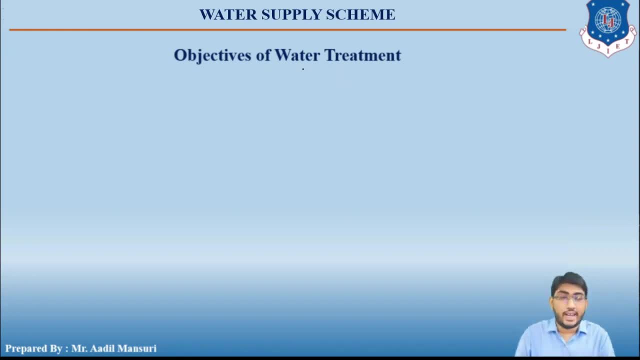 it should be and it so that it is aesthetically attractive, okay, and these, all these treatments should be done in economical manner, okay. next is water treatment. processes are basically meant for removal of impurities, or impurities of water, so this is the main aim of water treatment. 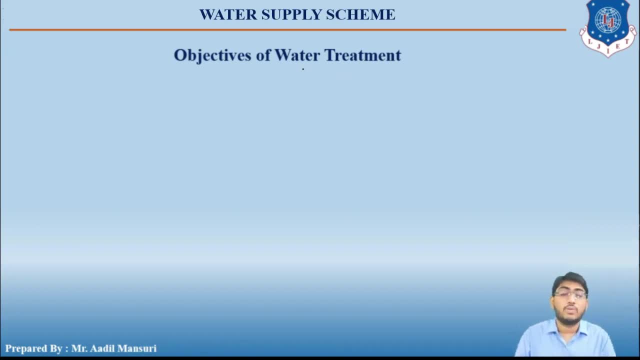 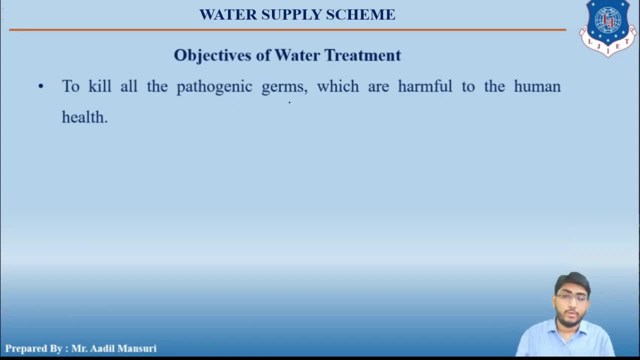 organisms before supplying the water to the community. Next is to remove the unpleasant and objectionable taste and odors from the water. So we know that when we extract water from different sources there are chances that there may be some decayed animals or decayed dead bodies of 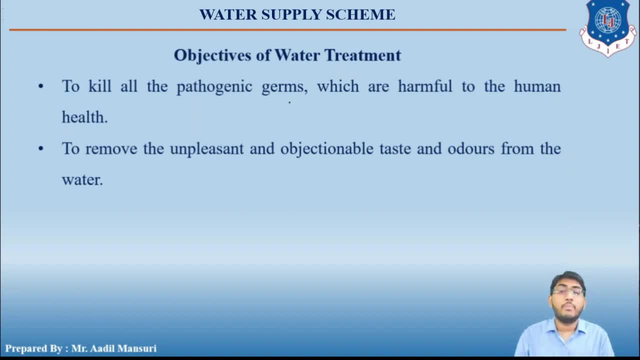 human beings present in the water, which will impart unpleasant and objectionable odors or taste right. So it is necessary to remove these unpleasant and objectionable taste and odors from the water. Next is to remove the dissolved gases and murkiness and color of the water. So we know. 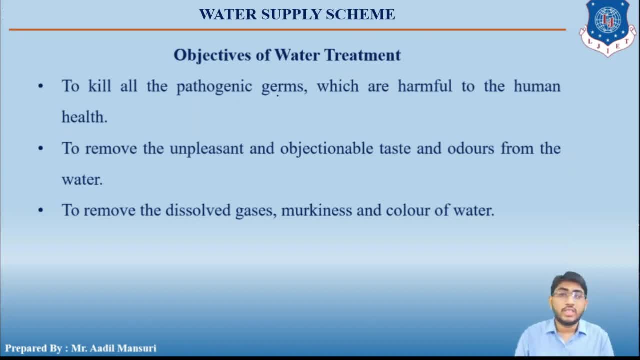 that sometimes these sources are connected illegally by the industries and, as a result, what happens is sometimes these industries dump their industrial waste water into the these sources, resulting into imparting the colors to the water. Okay, so we need to remove all these colors, murkiness and the dissolved gases. Okay, next is to make water fit for domestic, industrial 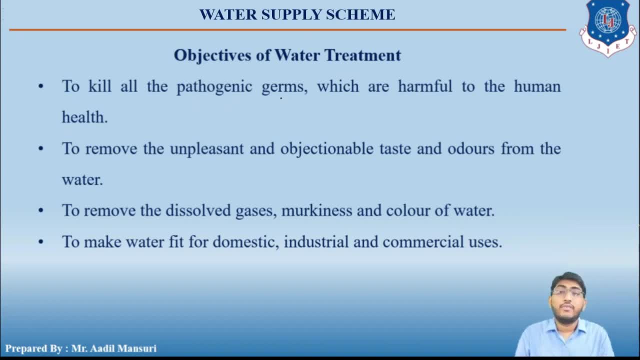 and commercial purpose. So after treatment you should check whether the water is capable for using in the domestic or industrial or commercial uses or not. Okay, Next is to eliminate the tuberculative and corrosive properties of water which affect the conduits and pipes. Okay, so we know that in the water 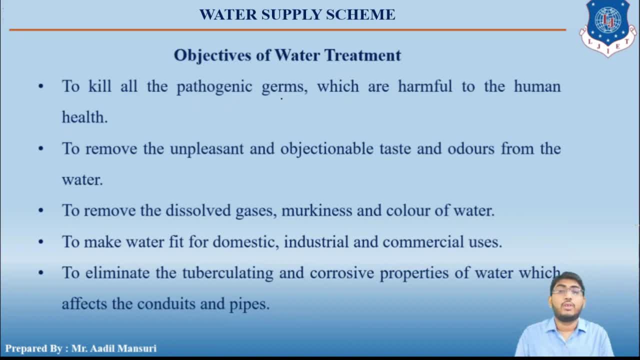 there are chances of components of recomendable subscribers presence of components of iron. these components of iron have the corrosive properties and that may lead to corrosion of the conduits. so we should take care of the thing that all the corrosive properties and tuberculative properties should be removed. 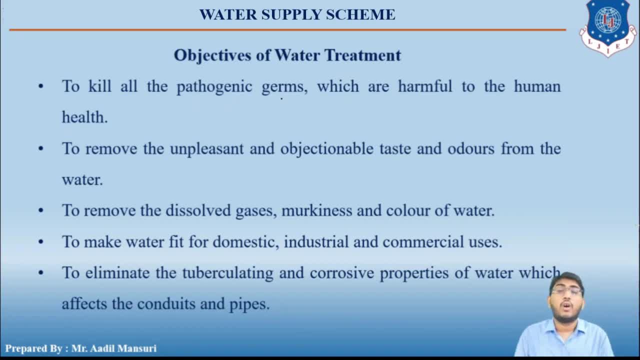 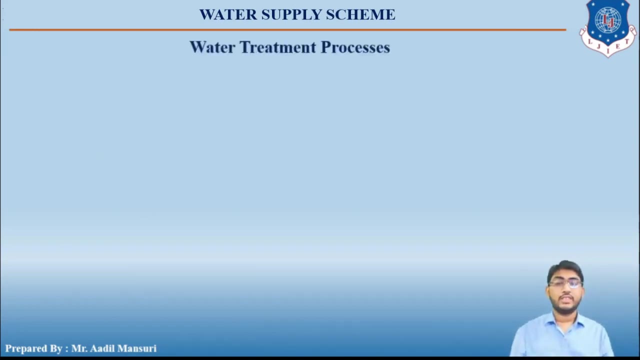 while the water is transferred or it is supplied with the help of conduit. okay, so these are the different objectives of the water treatment. okay, students, so let us now move towards the next topic, that is, the water treatment processes. okay, so, in a water treatment plant, there are various processes. 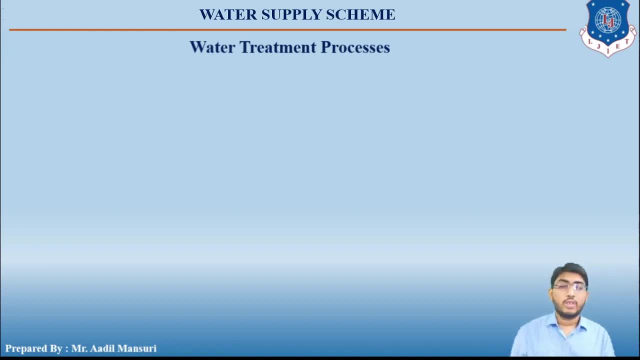 for removal of different types of impurities. so let us have a look at it one by one. so the first treatment process or treatment unit is known as the screening, then plain sedimentation, then sedimentation aided with coagulation, then filtration, then disinfection, aeration. 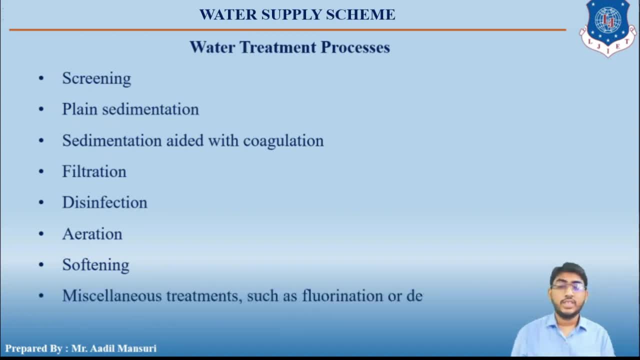 softening and other miscellaneous treatments such as fluorination or desalination. okay, so what are the functions of each of this? okay, so floating matters like tree leaves or branches, pieces of papers, fishes or other lightweight materials are removed in screening process. okay, next is plane sedimentation, so the suspended matters having higher specific gravity than the water, and which 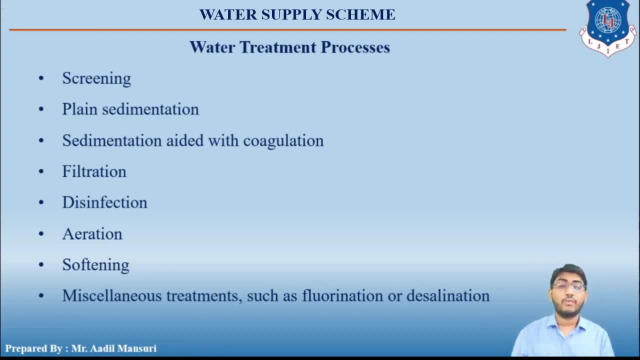 are able to settle under the effect of gravitational force in still condition. right, and those metals are, or those matter are like pebbles or aggregates or horse sand, etc. right, so these matters will settle down under the effect of gravitational force. right, so this process of removal of these matters is known as the plane sedimentation. okay, next is sedimentation. 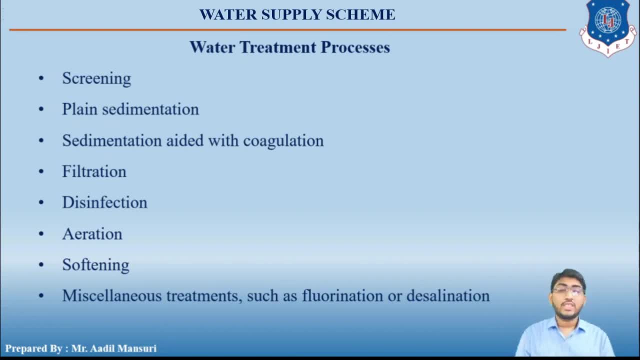 so the plane sedimentation. it is the process of removal of the material from the surface of the ocean and it is under the effect of gravitational force. that is the plane sedimentation, added with coagulation. so so fine suspended matters such as clay, silt, fine sand etc. will get removed by 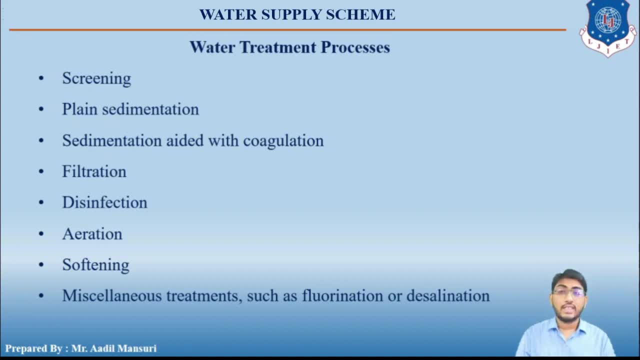 addition of an external chemical which is known as coagulant. okay, so what will happen is that, due to, they will group together and, because of the increase in weight, they will settle down. so this process is known as sedimentation aided with coagulation. okay, next is microorganisms. 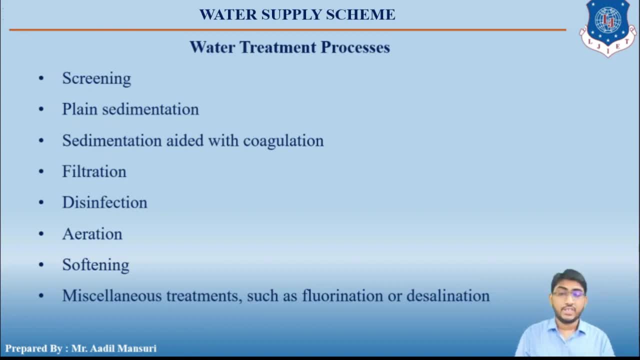 and colloidal matters will be removed in filtration. okay then, in case of aeration and other chemical treatment, we can remove dissolved gases taste or odors. okay then, in case of water softening, we will be able to remove hardness. okay, so we know that sometimes, when you 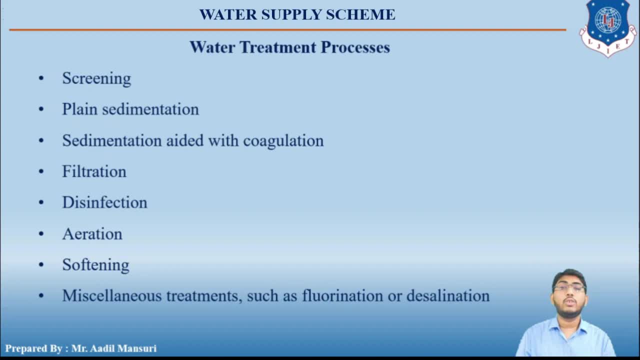 add detergent to water, then it is unable to produce the froth. okay, this is because of the hardness property of the water. okay, so we need to remove the hardness, which is done with the help of softening. there are various processes for removal of hardness. okay, next is chlorination or 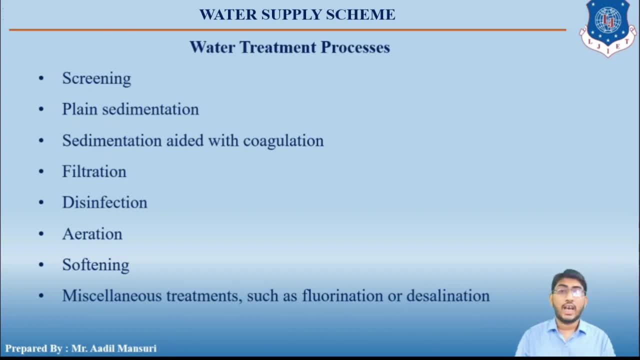 disinfection in which pathogenic organisms are removed. okay, so the type or degree of treatment to be given to the raw water will depend upon the nature of water or the source of the water. okay, if the surface source of water is available, all the above types of treatment. 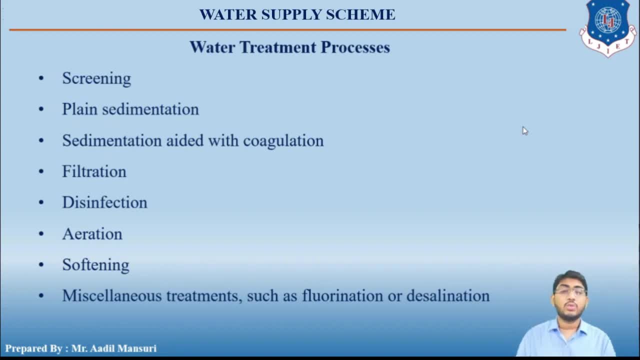 processes should be employed, and if the source of water is like lake or impounding reservoirs, then water is free from suspended matters and it will require only filtration or disinfection. right ground waters are usually clear, so only disinfection may be done, or sometimes even disinfection is also not required. okay, sometimes they required softening. 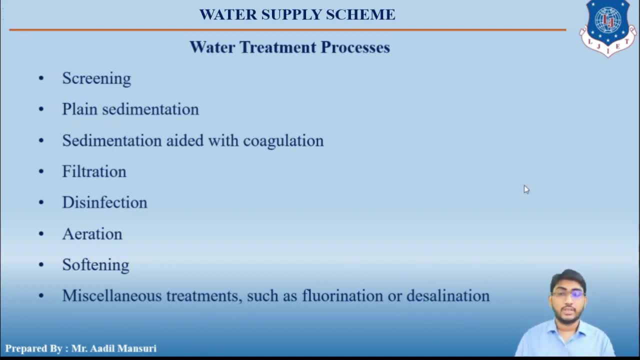 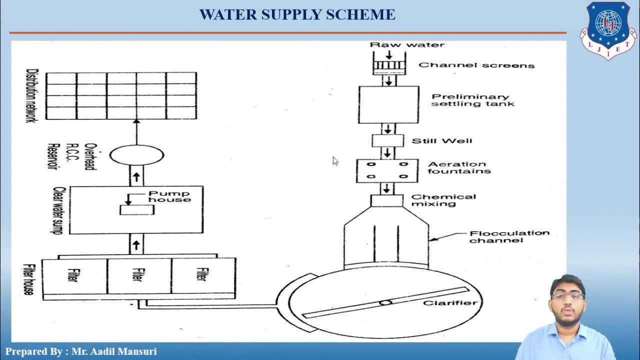 and chemical treatment for removal of minerals. okay, so this is the layout of the water treatment plant. okay, so it will start from the raw water, right, then this channel screens where all the floating particles will be removed. preliminary settling tank where all the suspended particles will remove under the effect of gravity, then steel, well then aeration fountains in which 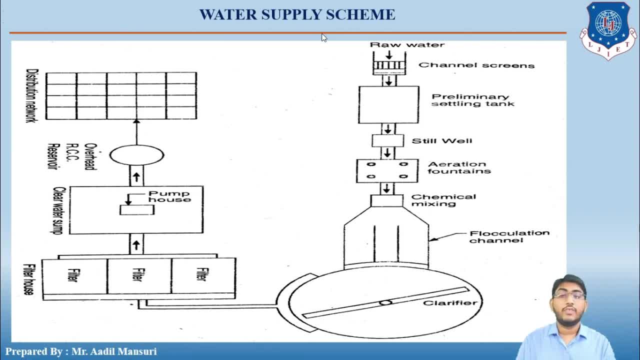 these will address the seedlings that are located in further surface and this addition of these hosting factors will put them down. the gladiator miał gas element: these anything containing nitrogen from contaminants used in Sócia inNão heraus to the cloud. the liquid of the first layer will next mix the algum material taken. 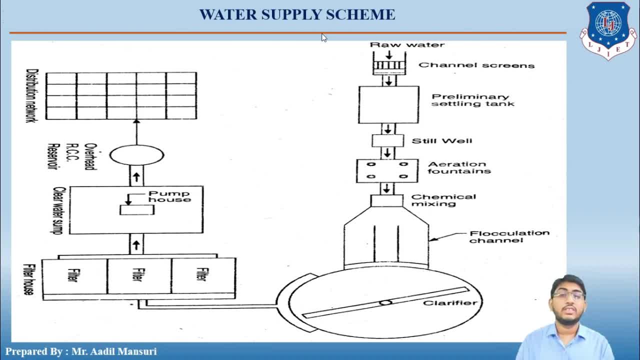 acid, which is which excrete the salmonella. it basically would form of magma which would be combined with a gas, but the react in those things, that is, every plant of fedora Insase would and complex, and the gaseous, which is exactly the same as an enol. 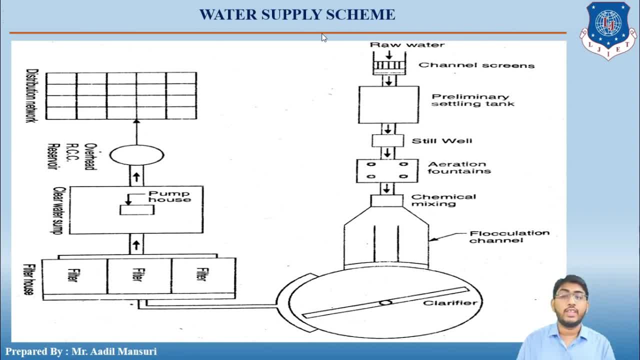 will not go through these niches by itself, So there will be a coke like case. every bike size machine will begin to conduct it. so, aki place injection, the water will be Rincon, Alexandre Manteau, depending on the how to go about it in Filtern 버� unglaubweiss. 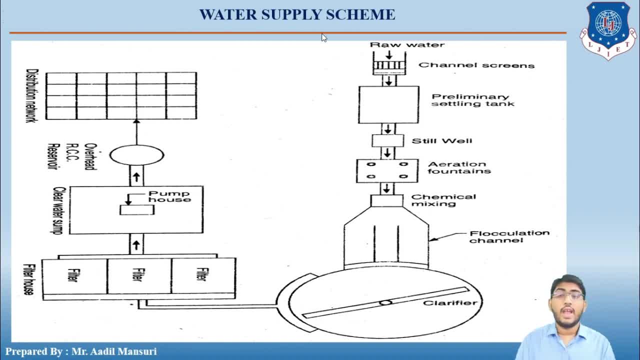 after the filtration, water is stored, and about there there is a pump house which is supplying the clear water to a particular area overhead reservoir, and then it is distributed to the community. so this is how the complete layout of the water treatment plant is okay. so let us now. 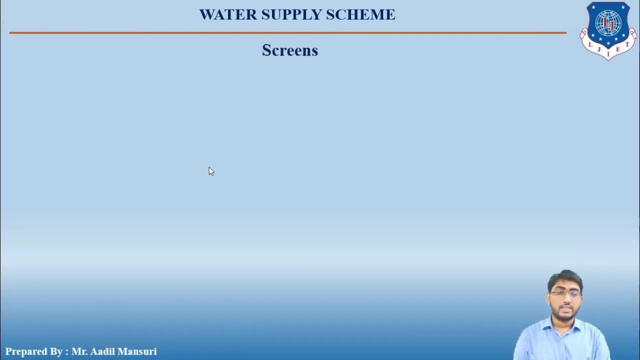 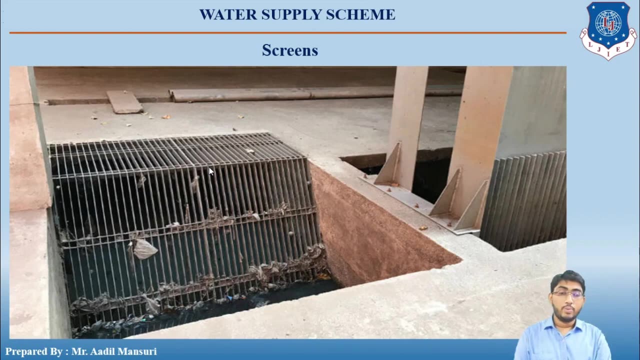 move towards the next topic and that is the screens. okay, so you can see on the screen these. there is a screen, so there is an open channel under the screen and you can see here that the floating particles are trapped before going inside the water treatment plant. okay, so, 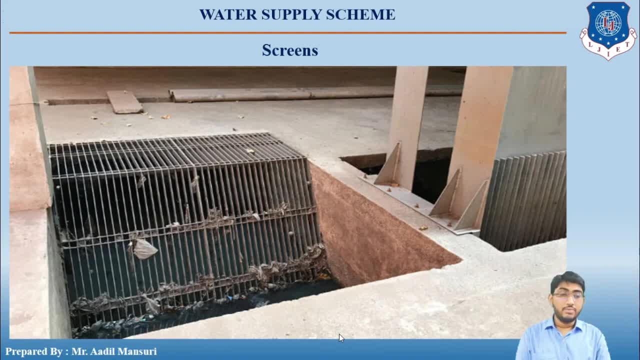 screens are generally provided in front of the either pumps or intake pulse, so to exclude the floating and large size impurities such as leaves, branches of trees, aquatic vegetation, fish, ice, etc. So core screens, which are also known as the trash racks, are also sometimes placed in front. 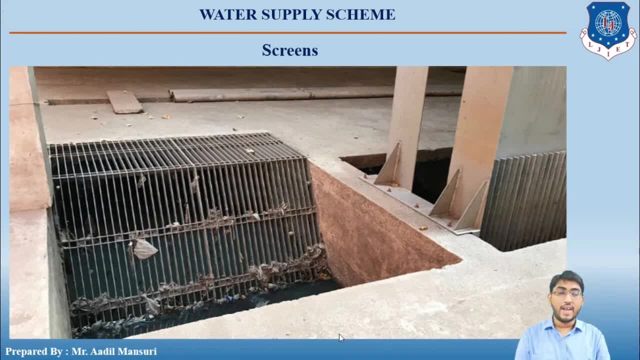 of the fine screens. Core screens consist of parallel iron rods placed vertically or at slope at about 2-10 cm center to center. The fine screens are made up of wires or perforated metals with opening less than 1 cm wide And the core screens first. removes the bigger floating particles and the fine screens removes. 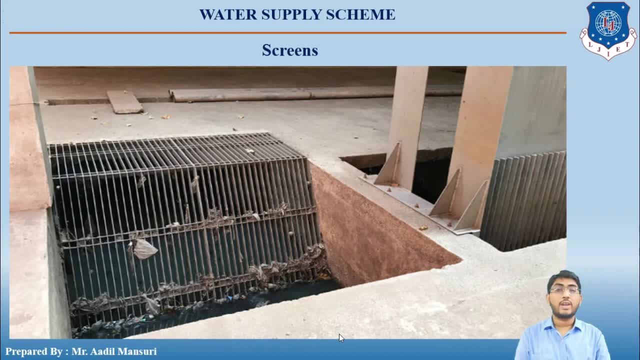 the fine suspended solids. So there are total two types of screens, that is, core screens and the fine screens. Clear students Now. the fine screens normally gets clogged and hence required to be cleaned frequently. The fine screens are therefore avoided and the fine particles are separated in the sedimentation. 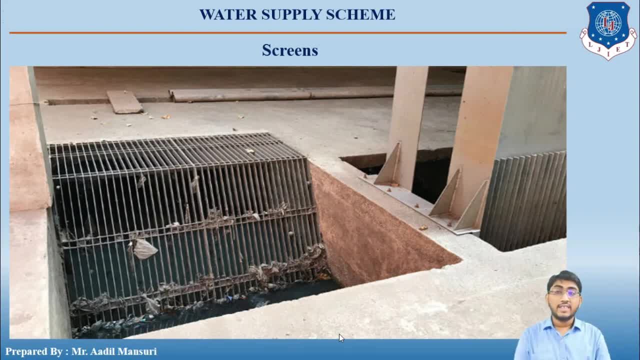 So the fine screens normally gets clogged and hence it needs to be cleaned frequently, And the fine screens are therefore avoided and all the fine suspended particles are removed in the sedimentation. Now the core screens are normally kept at an inclination of 45 to 60 degree, with the 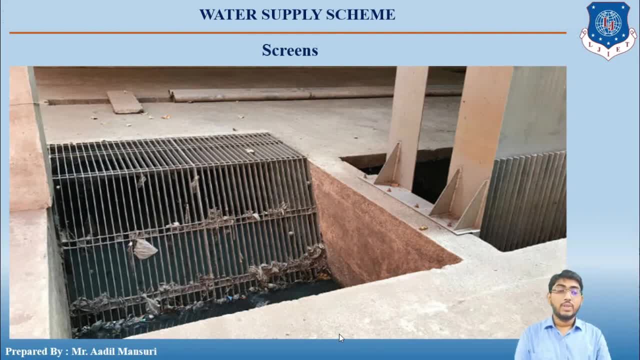 horizontal and so that this will increase the opening area and reduce the flow velocity. Right So this will make the screens more effective. So here in the picture you can see that the screen is at an angle, right So it is at. usually the screens are placed at an angle of 45 to 60 degree, with the horizontal. 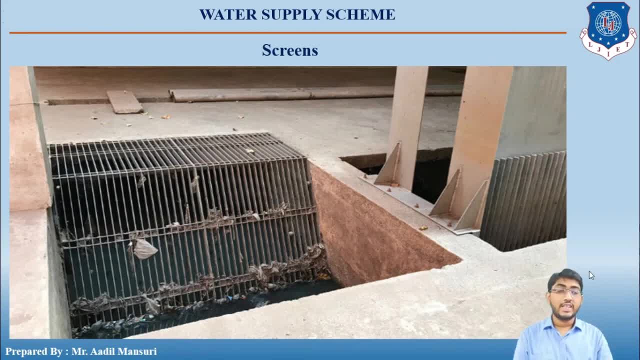 Okay, students, Now, while designing the screens, clear openings should have sufficient total area so that the velocity through them is not less than 2 cm. Okay, students, Then. 0.8 to 1 meter per second, right, So the flow velocity of the screens should be kept minimum: 0.8 to 1 meter per second. 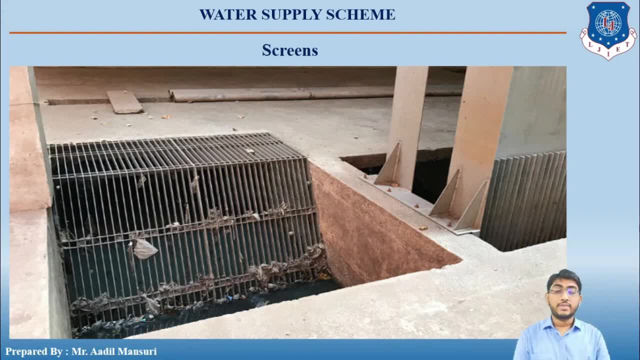 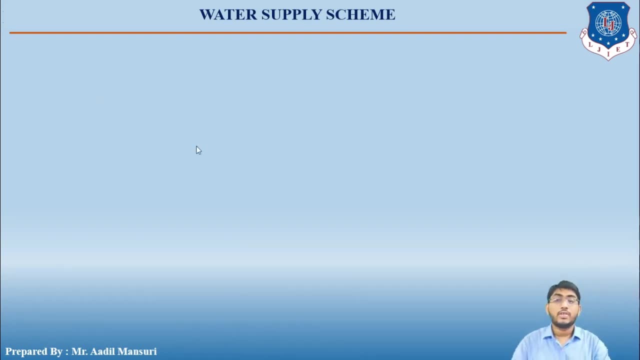 And the material which is collected on the upstream side of the screen is either manually or mechanically removed. Okay, students, So this was about the screens Clear. Okay, students? Okay. So let us now have a look at the new topic, that is, the plane sedimentation. 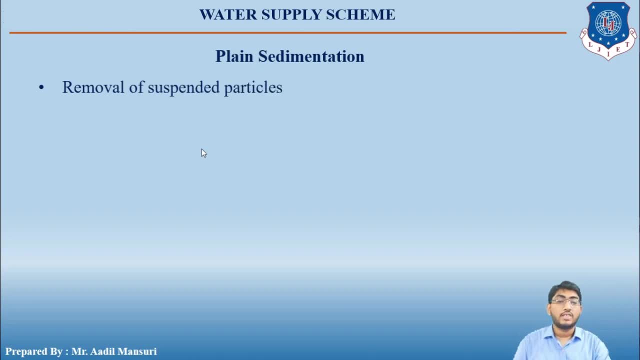 Okay, So sedimentation is the removal of the suspended particles by gravitational settling. Okay, By definition, sedimentation is a solid-liquid separation using gravity settling to remove suspended solids. Okay, Most of the suspended solids present in water possess specific gravity greater than that. 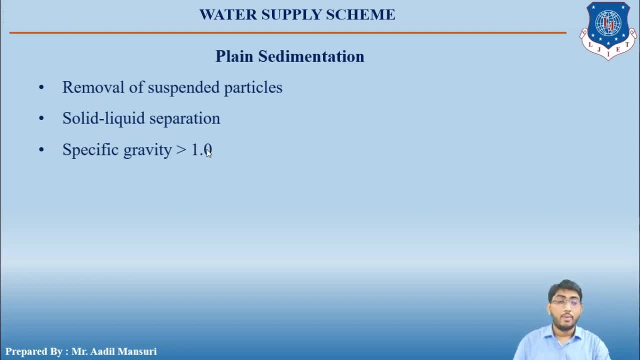 of the water. That is water. Okay, Now, these particles are held in suspension due to turbulence in the water. When this turbulence is retarded by offering the storage of water right then the suspended matter tends to settle down at the bottom of the tank. 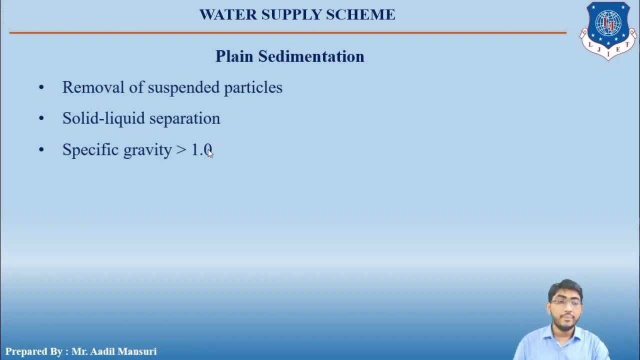 And this is the principle behind sedimentation, Understood students. Now, the basin in which the flow of water is retarded is called the settling tank, or sedimentation tank, or clarifier, And theoretical average time for which the water is stored in this tanks is known as. 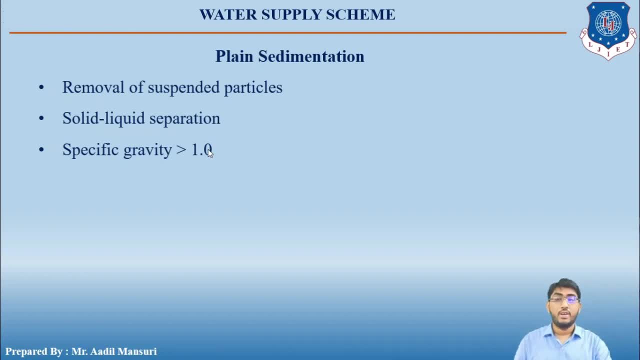 the detention time or detention period. Okay Now. sedimentation tanks are designed to reduce the velocity of flow of water so as to permit settlement of the suspended solids by gravity. Okay, So we will be looking at the various types of sedimentation tanks. 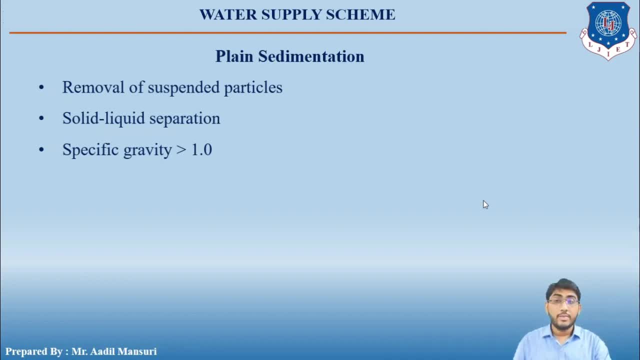 Okay, So the main function of the sedimentation tank is to reduce the velocity of the flow so that all the heavier particles will settle down at the bottom. Okay, And main application of the plane sedimentation is to remove heavy settlable solids from turbid. 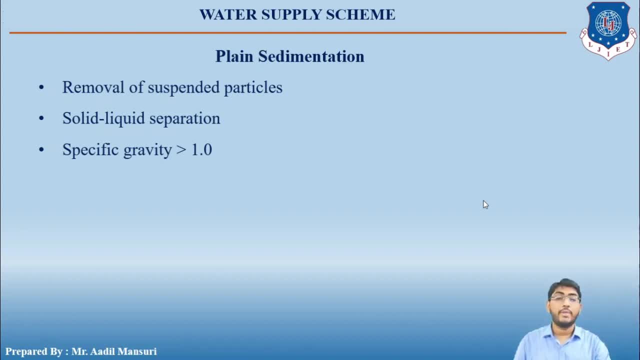 source to lessen the solid load on the treatment plant processes. Okay, Because the sediments are removed from the water, then the load on the successive treatment units will be reduced. As a result, the efficiency of the successive treatment units will increase. Okay. 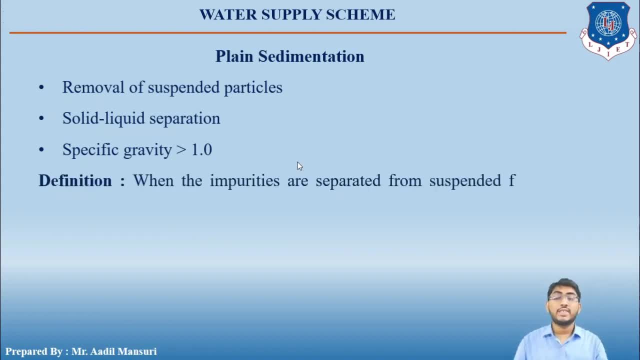 So once again, let us have a look at the definition. When the impurities are separated from the suspended fluid by action of natural forces alone, that is, by gravitation and natural aggregation of settling particles, then the operation is known as plane sedimentation. 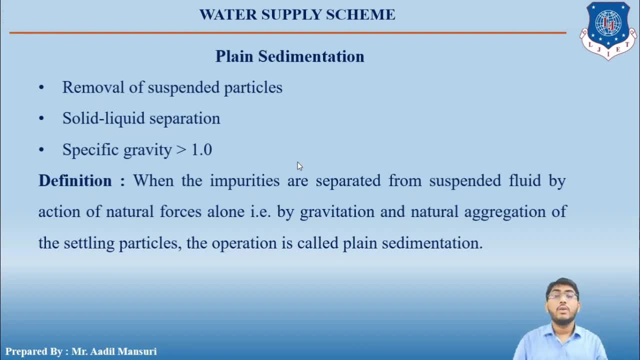 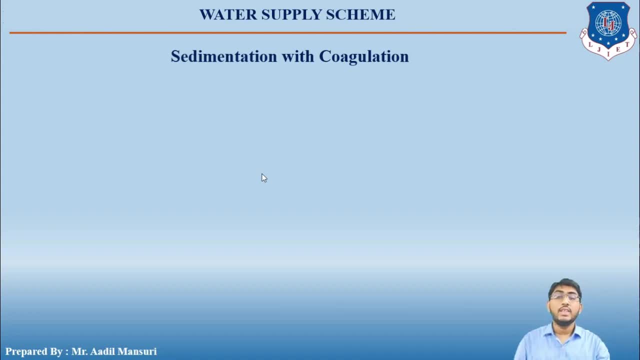 Understood students. So this is the theory of plane sedimentation. Let us now move ahead. Let us now have a look at the topic sedimentation with coagulation. Okay, So when chemicals or other substances are added to induce or hasten or to increase the 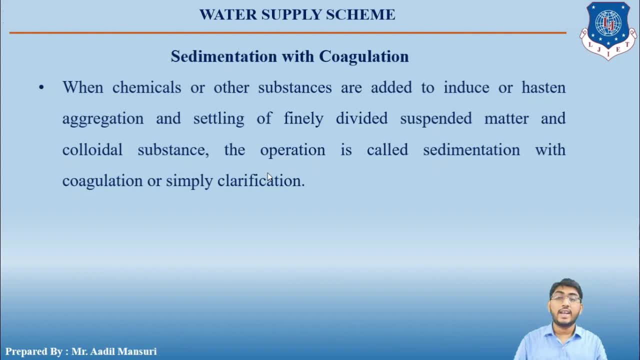 speed of aggregation and settling of finely divided solids, Finally divided suspended particles and colloidal substances. Then the operation is known as sedimentation with coagulation, or simply clarification. Okay, So once again, when all the suspended particles which are not settling in the plane sedimentation, 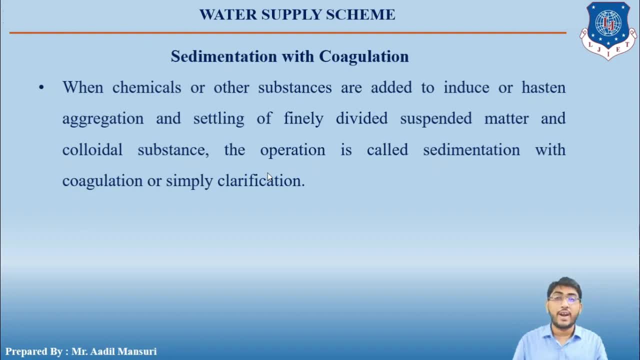 then these set- this set suspended particles will remove- will remain in continuous motion, Right. So, in order to remove those suspended particles, We need to add a certain chemical or other substances in order to gather those particles, to increase their weight and to make them settle at the bottom of the sedimentation. 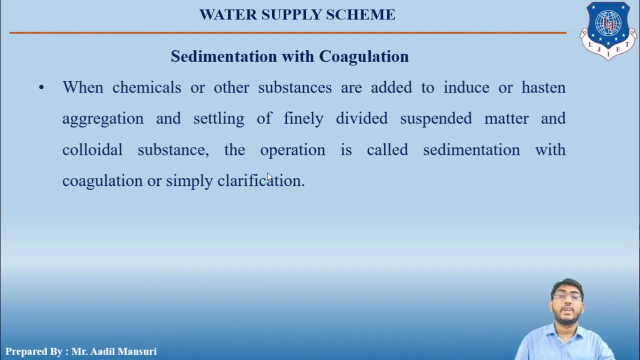 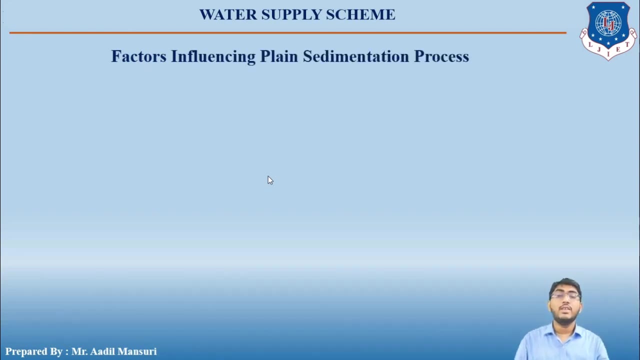 type. So this phenomena is known as sedimentation with coagulation. Okay, So one of the most famous coagulant is the alum. Okay, students, Let us now have a look at the next topic, That is, the factors influencing plane sedimentation process. 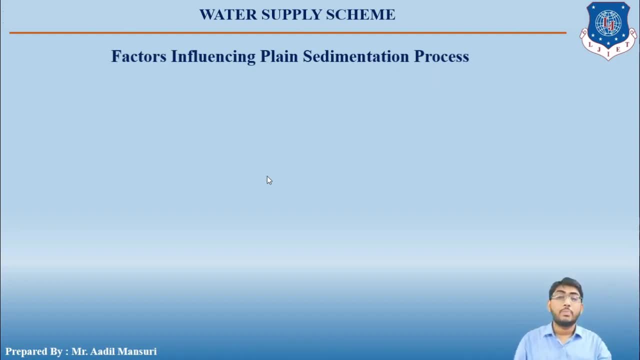 Okay, So there are various factors on which the plane sedimentation process depends, For example, size, shape and weight of the particle. If the particle will be more in size and it will have more weight, then the particle is going to settle at more faster rate compared to the particles of smaller size. 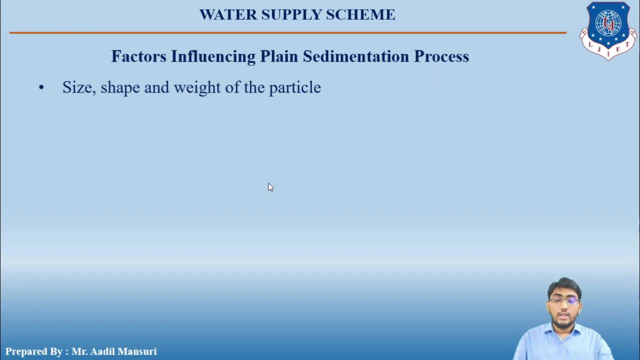 And lesser weight. Okay, next is viscosity and the temperature of the water Right. Third one is the surface overflow, Then is the velocity of the flow. If the velocity of flow will be more right, then it will get less time for the settlement. 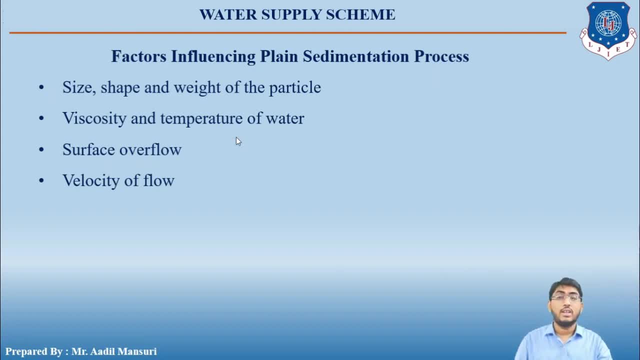 Hence the particles will not settle easily. Okay. Next is inlet and outlet arrangement, Then detention period: Okay. if the detention period is more, then the efficiency of sedimentation will be more okay. next is effective depth of basin: okay, and last is the surface area. so these are the factors which 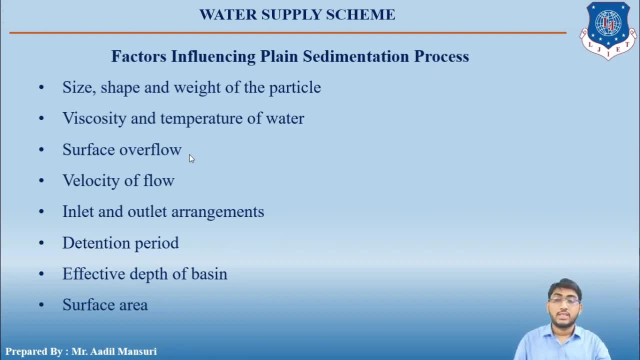 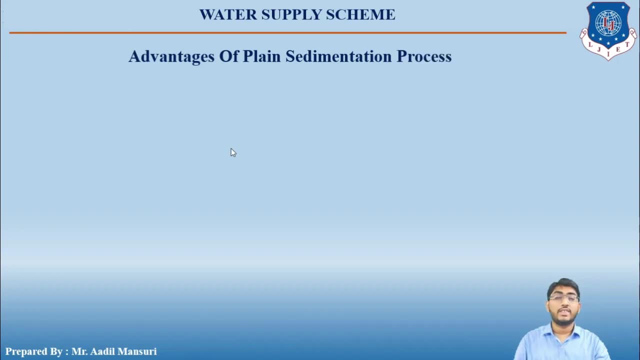 influence the plane sedimentation process. okay, students. so let us now have a look at the next topic, that is, the advantages of plane sedimentation process. okay, so it lightens the load on this subsequent process. okay, so, for example, if you don't carry out the sedimentation process, then 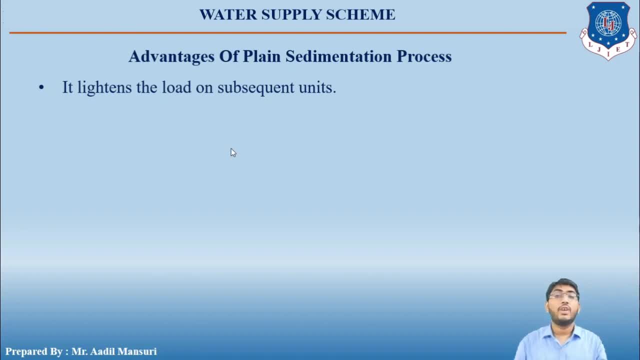 what will happen is, in the filtration process, the filters will get jammed. okay, so as a result, the efficiency of filters will reduce. right? so if you do the sedimentation process, then the load on the subsequent units will be lessened. okay, then the operation of the subsequent process. 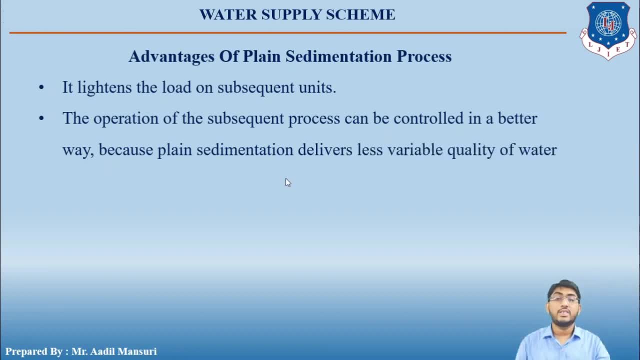 can be controlled in a better way because plane sedimentation delivers less variable quality of water. okay. next is less quantity of chemicals are required in the subsequent treatment process. okay, so if the plane sedimentation process is done properly, then the less chemicals will be required for the subsequent units. the cost of cleaning the chemical coagulation basin is reduced. 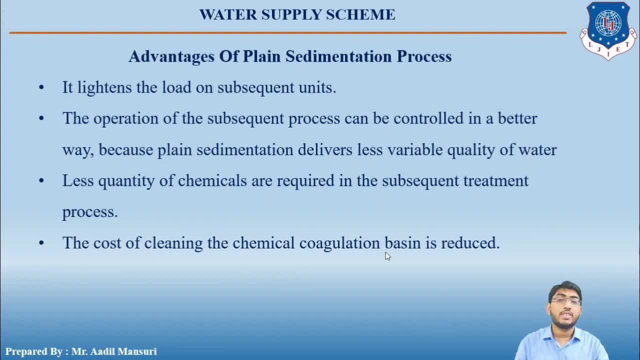 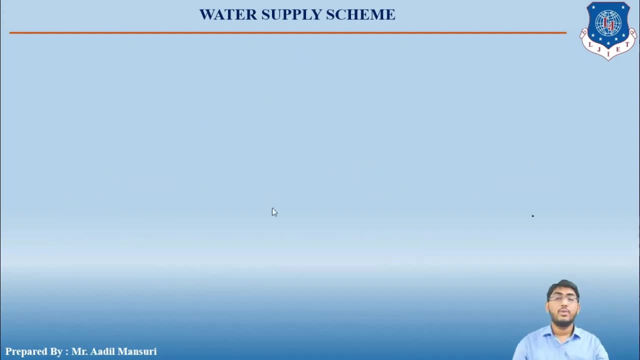 right, because majority of these suspended particles are removed in the plane sedimentation. next, no chemical is lost with sludge discharge from the plane settling basin. okay, so let us now have a look at some of the important terms, and the first term is the. is the coalesce, right? so the meaning of the coalesce is to come together, right? so when you 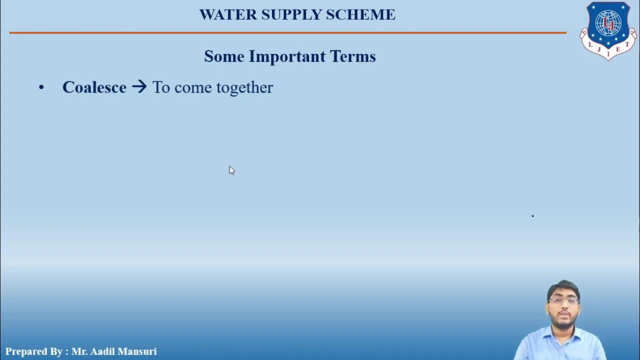 add chemical like coagulant into the water. what will happen is those particles which are heavier will settle down, but which are not able to settle down and which are moving constantly. what will happen is, due to the addition of coagulant, those particles will come together and this phenomena 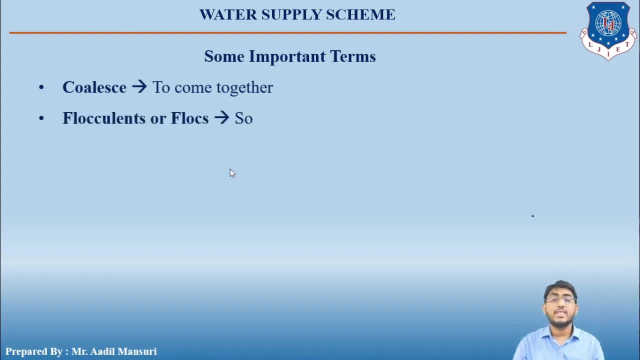 is known as coalesce. okay, next is flocculants, or the flocks. so when you add chemical to the water, the those particles which have come together will settle down at the bottom of the tank and these particles will have soft wool like texture, right, and those particles 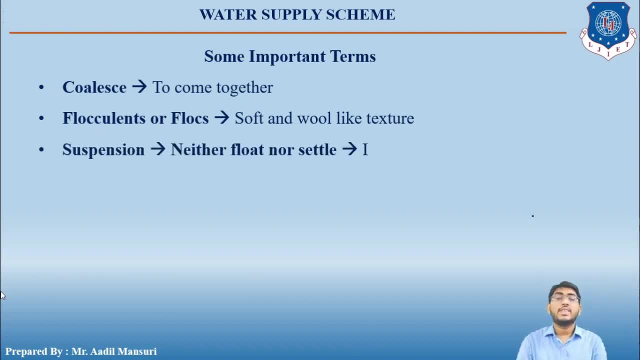 are known as the flocks. okay, next is suspension. so the meaning of suspension is that the particle will neither settle nor it will float in the sedimentation tank. however, it will remain in continuous motion. okay. next is the discrete particle, so a particle which does not alter its 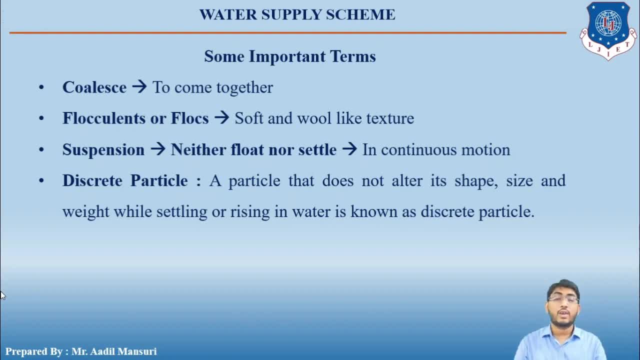 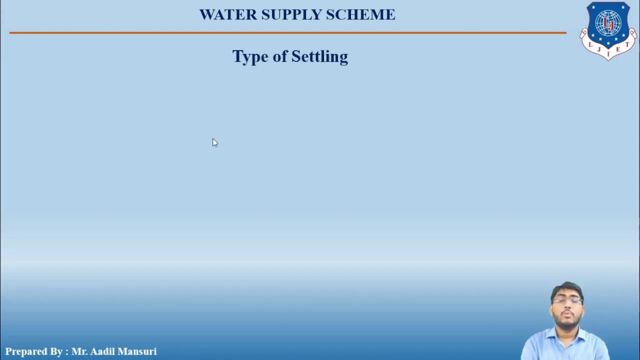 shape, size and weight while settling or rising in the water is known as the discrete particle. okay, so, these are the few terms that you should keep in mind for the upcoming theories. okay, so let us now move towards the types of settling. okay, so, basically, there are four types of settling. 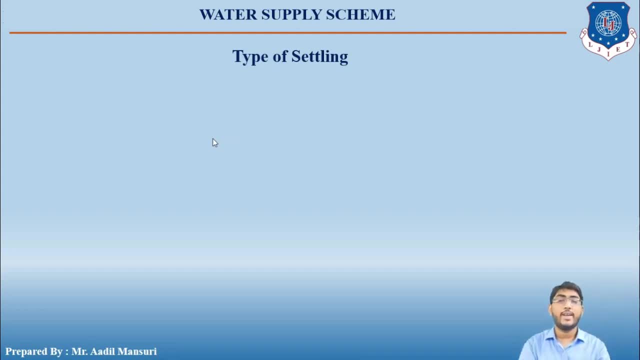 type one settling, type two settling, type three settling and type four settling. okay, type one and type two refers to the water supply engineering, and type three and type four settling refers to the water engineering. okay, so let us have a look at it one by one. so the first type of settling, that is, 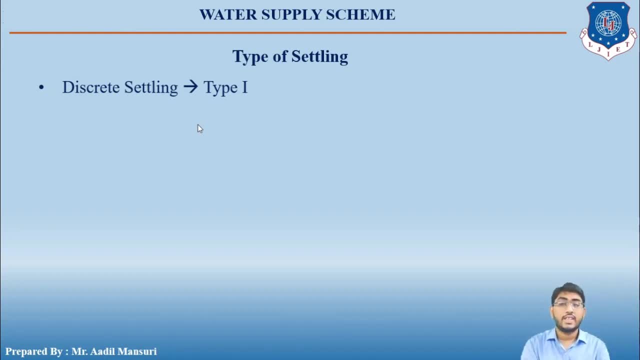 the type 1 settling. it is also known as discrete settling. okay, so discrete settling corresponds to the sedimentation of the discrete particles which are in suspension and in low concentration. okay, so this is also known as three settling, since these particles have little tendency to flocculate. 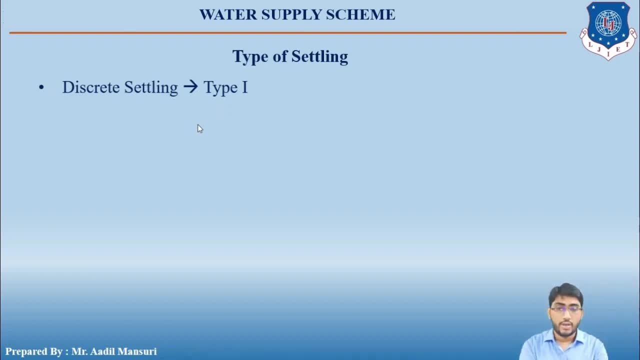 or coalesce upon connective shelters. so first it's called free settling, as these particles have little tendency to flocculate or coalesce upon contactousですね with each other. So these particles settle without hindrance to other particles, For example. 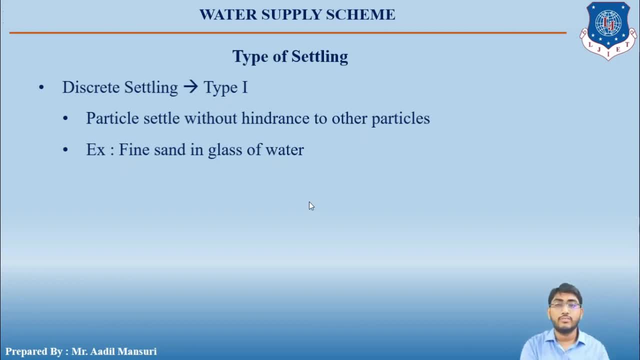 find sand in the glass of water. When you put some sand in glass of water, then they will show type 1 settling. Type 1 settling obeys Stokes law. Let us now have a look at the second type of settling, that is, type 2 settling, which is also known as the hindered settling. So 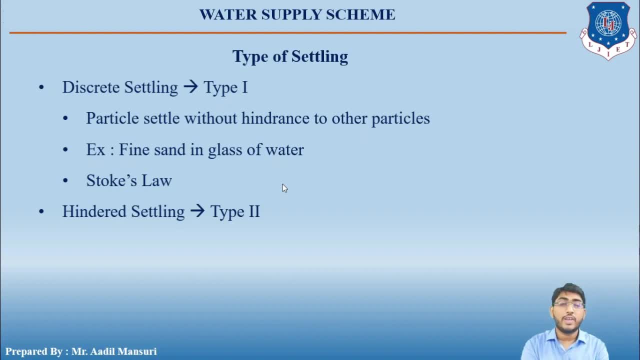 hindered settling refers to rather dilute suspension of particles that coalesce or flocculate during sedimentation process. Due to the flocculation, particle increases in mass and settle at the faster rate. This means that less particles in suspension and they will hinder 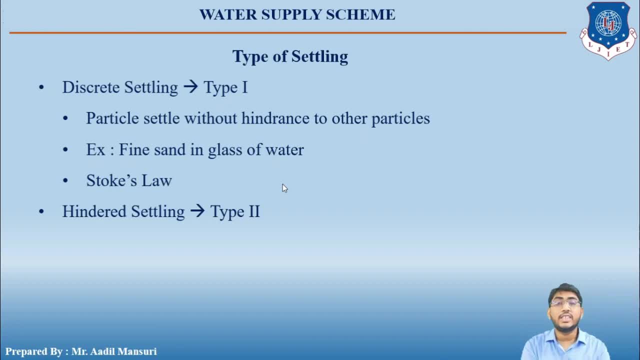 other particles while settling And thus increasing their mass. So in hindered settling the particles are in dilute concentration and they have less tendency to flocculate, But when they settle they increase in mass and settle at the faster rate. Okay, Let us now have a look at the third type of settling, that 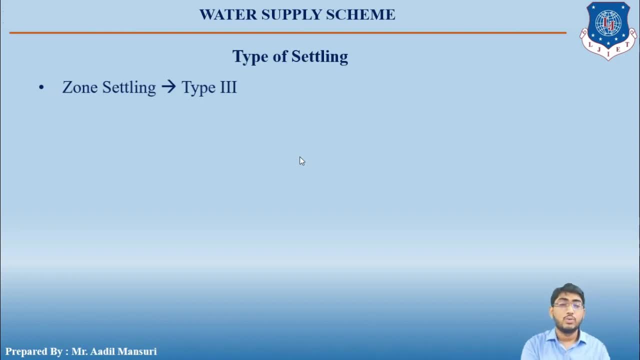 is known as the zone settling. Okay, This process mostly occurs after addition of the coagulants. So the zone settling refers to the flocculant suspension of intermediate concentration and interparticle forces hold the particles together and mass of the particles subside as the whole mass. Okay, So these flocculants are 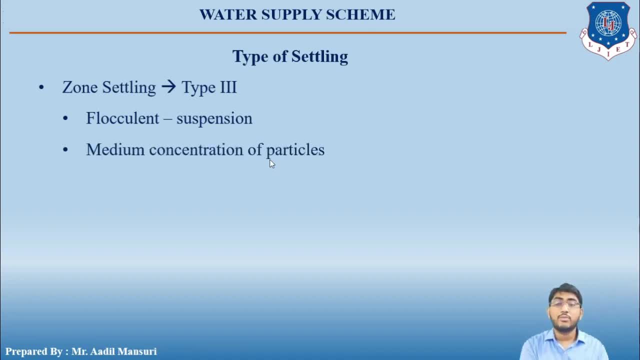 in suspension and they are in medium concentration, Okay. And these particles are hold together by a force known as the interparticle force. This will result in formation of mass and this will lead to increase in their weight. Thus, they will settle down, Okay. 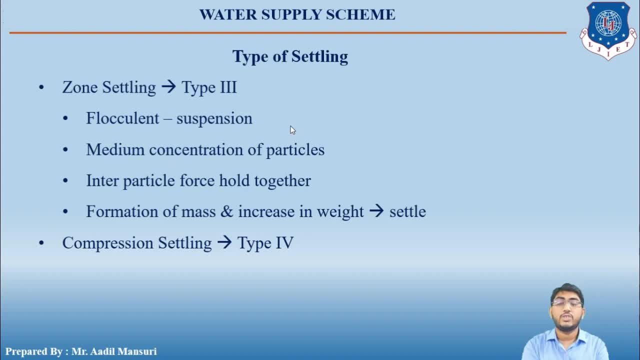 So let us now have a look at the fourth type of settling, which is known as the compression settling. So compression settling refers to flocculation, suspension of so much high concentration of the coagulant, So this is known as the compression settling. So this is.